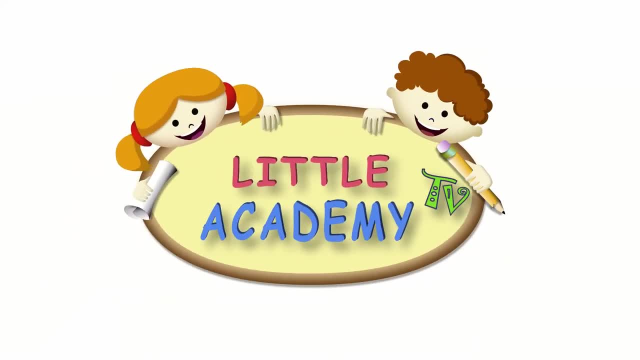 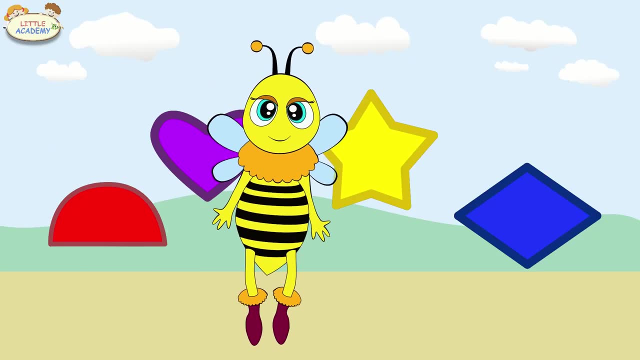 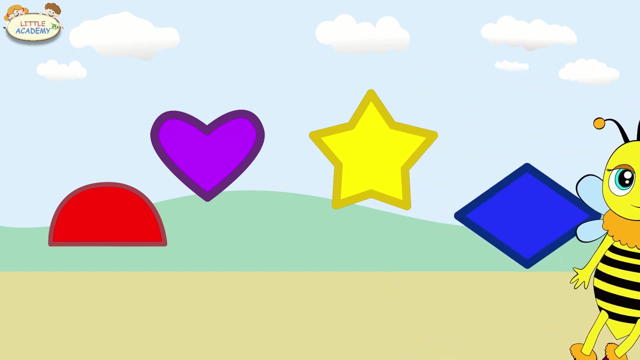 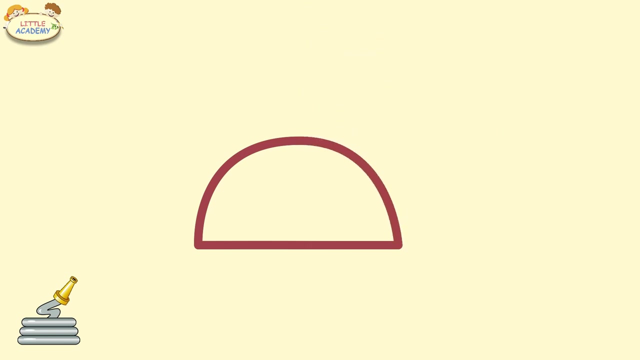 Hello, hello. Here is Polly the Bee again. Do you want to continue learning shapes together? Then let's go. RED SEMICIRCLE SEMICIRCLE, ORANGE SEMICIRCLE, SEMICIRCLE SEMICIRCLE, YELLOW SEMICIRCLE, RED SEMICIRCLE. 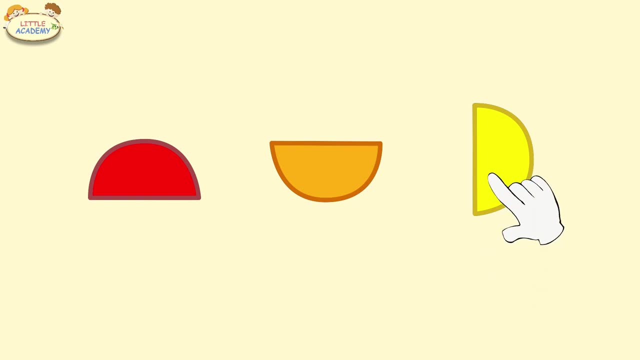 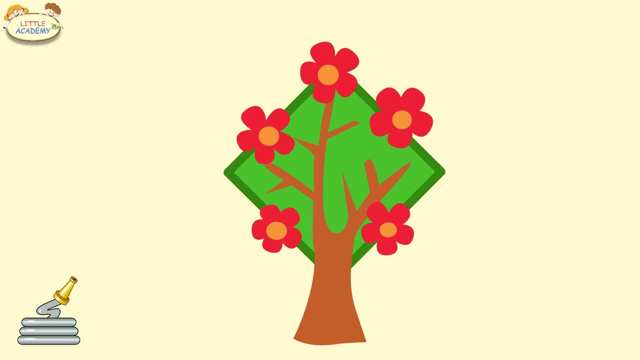 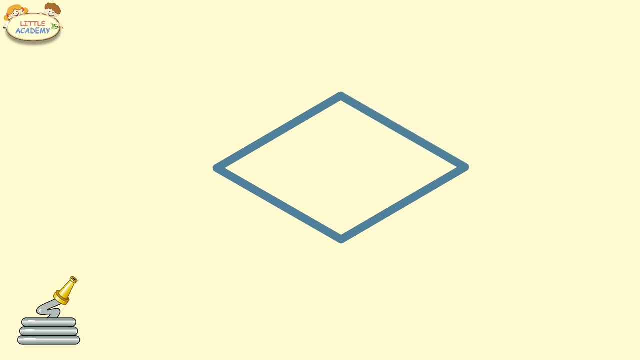 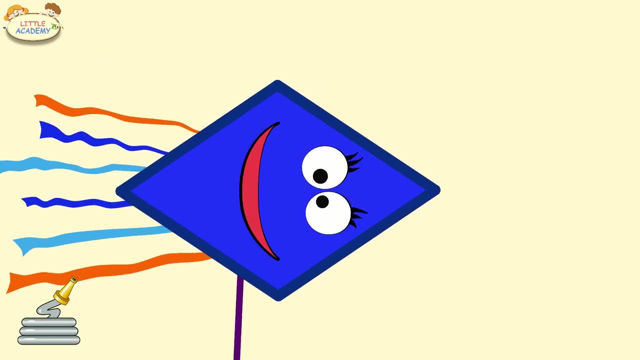 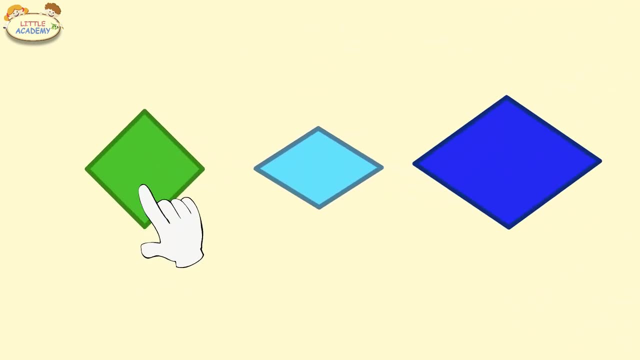 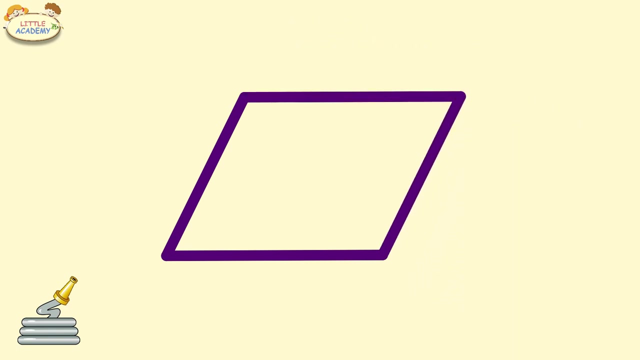 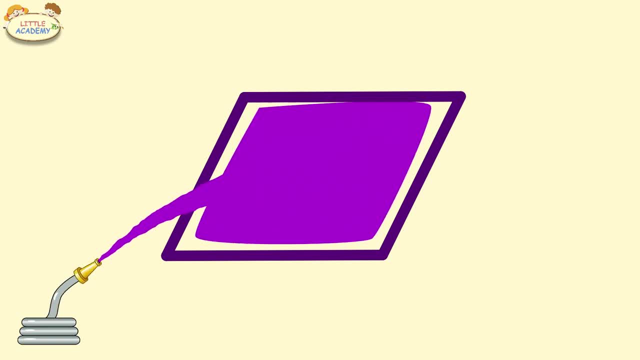 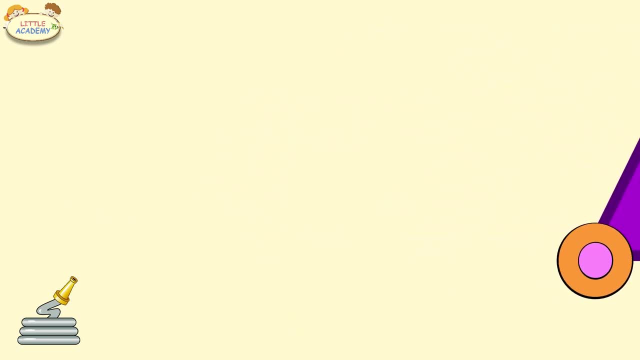 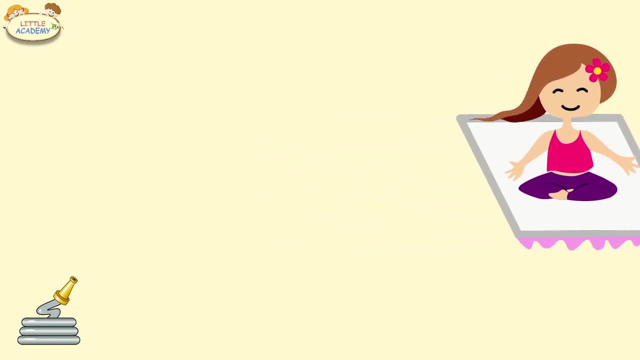 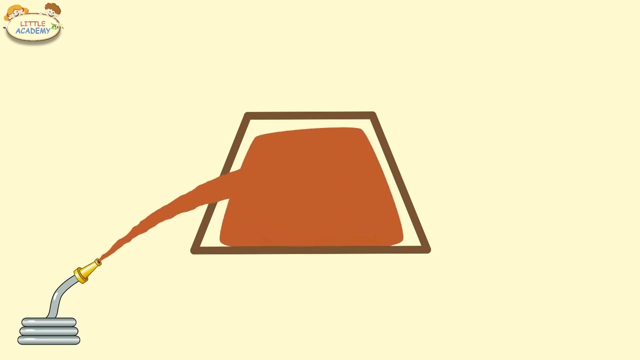 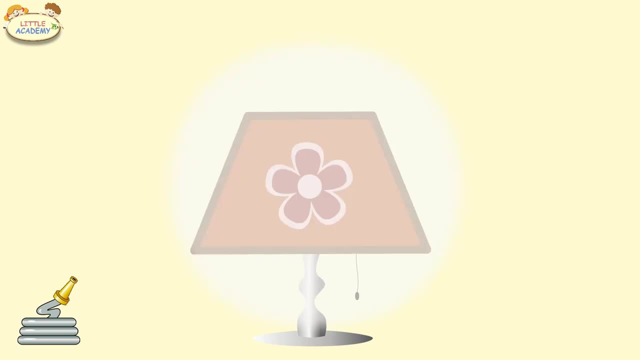 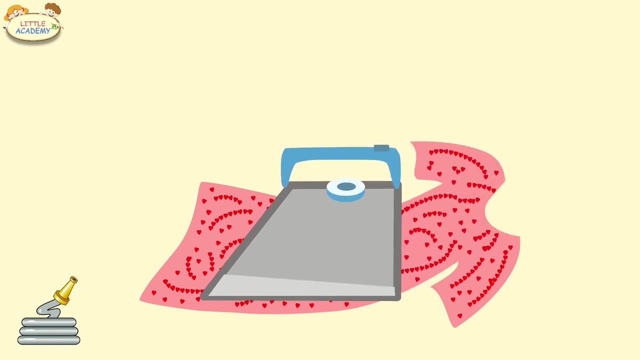 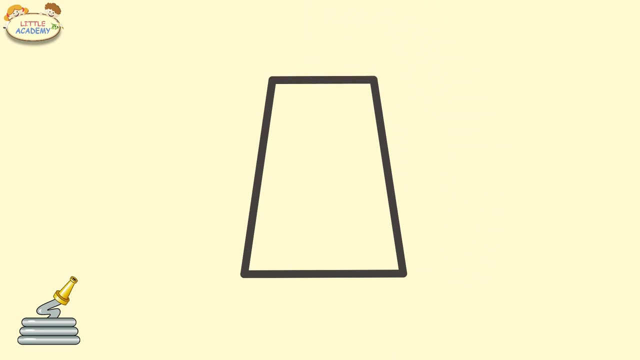 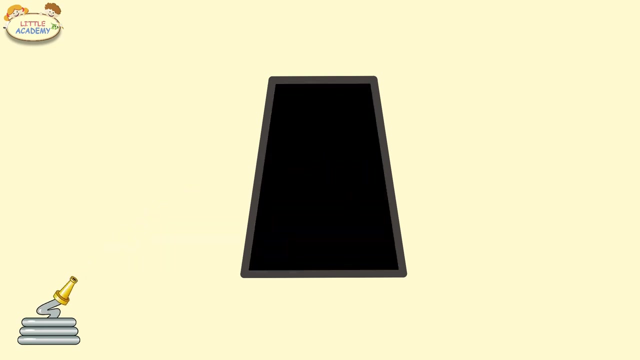 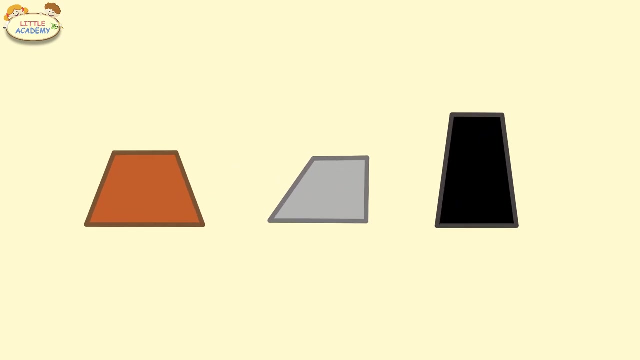 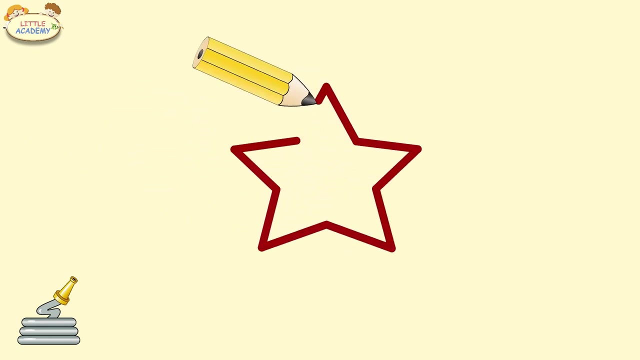 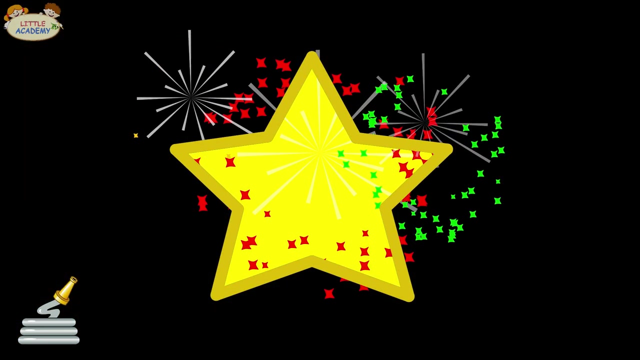 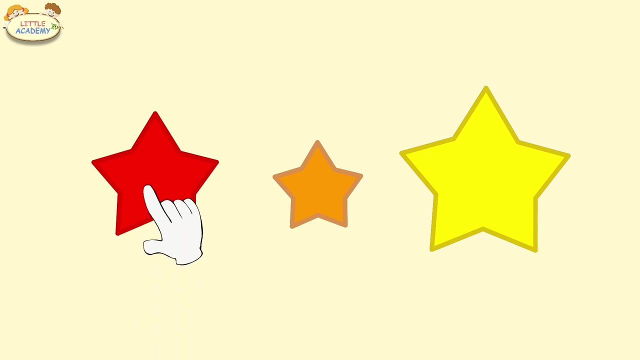 trapezoid grey trapezoid. trapezoid black. trapezoid brown. trapezoid gray. trapezoid black. trapezoid star red star. orange star. star star. orange star. star yellow star. red star. orange star, yellow star. 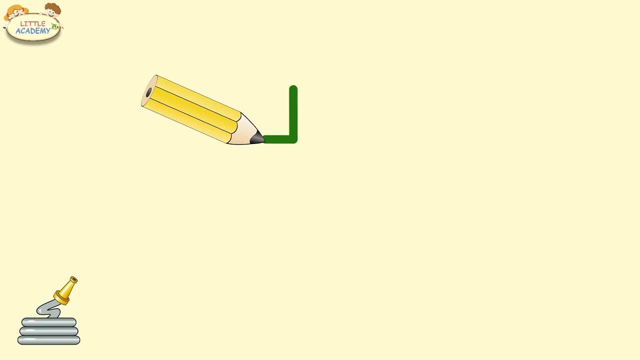 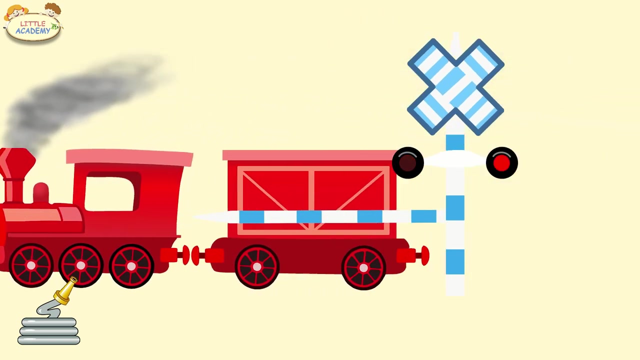 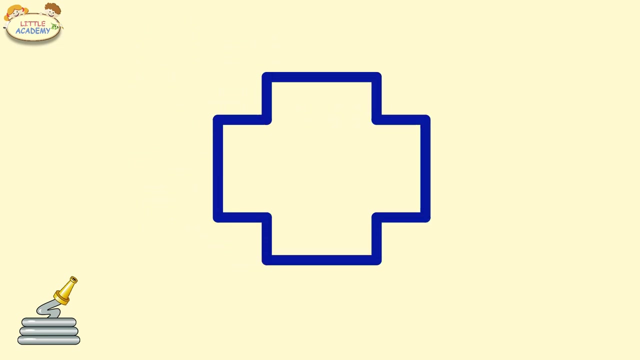 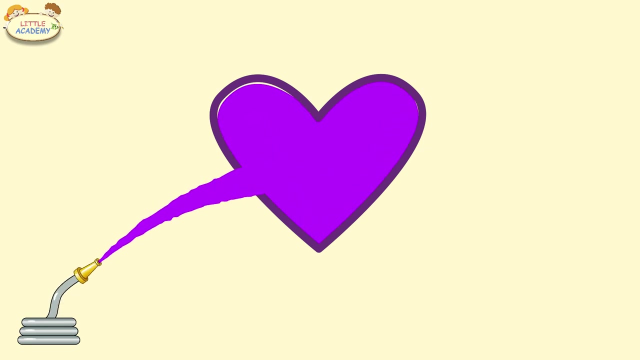 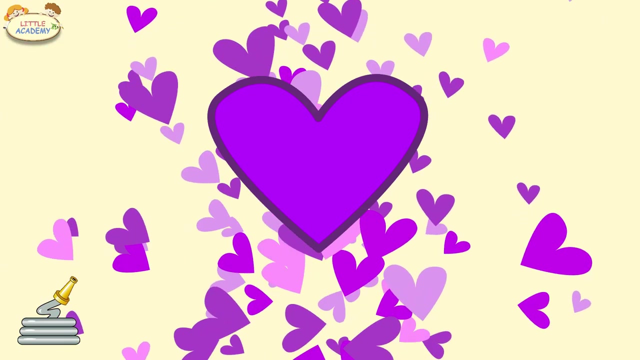 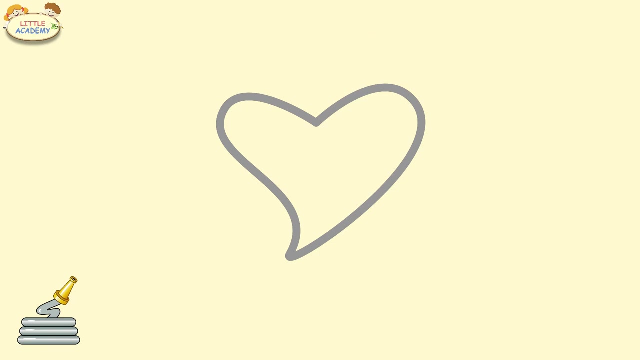 cross green cross. cross star white star. Liked blue cross. Cross Blue cross, Green cross. Liked blue cross, Blue cross. Heart Purple heart, White heart. Heart White heart. Heart, Pink heart, Purple heart, White heart.